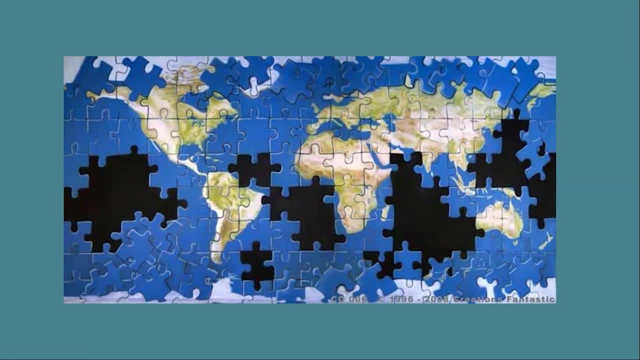 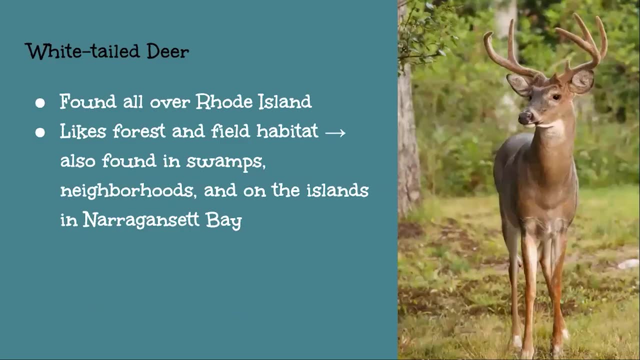 get kids thinking about: oh, what could this particular animal eat or be eaten by? So just a little introductory activity to get everything going for this lesson. So after the food web activity, there are two different games that you you can play, and you can play both of them, You could just play one of them. 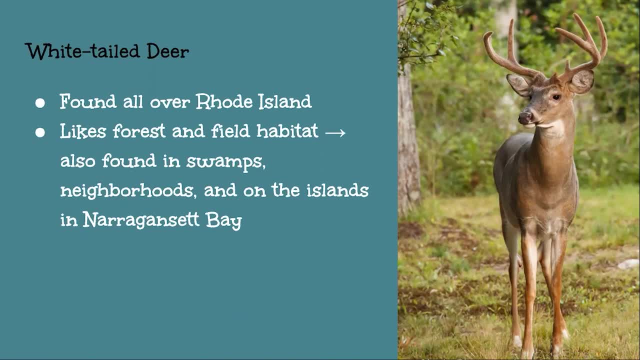 depending on the amount of time you have. One focuses on deer, the other focuses on perky, and they essentially say the same thing, you know. So wild populations respond to resource availability. So if there's lots of resources available for an animal, then we'll see our 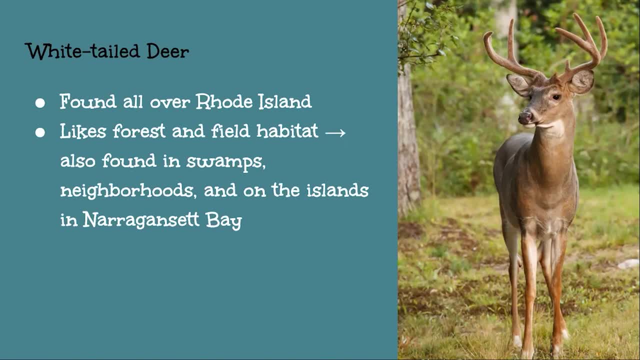 population start to increase. If there's not so many resources, we'll see our population start to decrease and we go through cycles And there's lots of different factors other than resources that will affect a population, like disease, like predation. 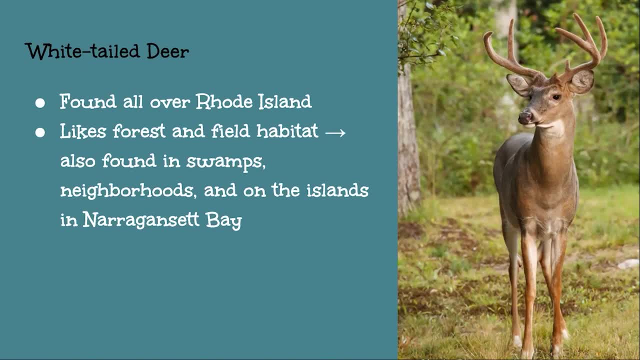 regulated hunting. So there's some fun ways that you can kind of manipulate the games to challenge kids to think about all of those different factors together. It's not just a kind of a cut and dry situation. It's very complex and they can start to think like a biologist. 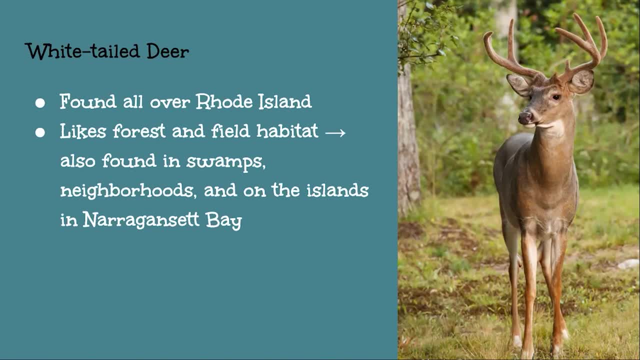 So before playing those games, we have some background information to learn about those, to get kids, using their imagination as they're playing the game, to think about all of the things that these animals go through in a particular year and seasonally, so that they can really 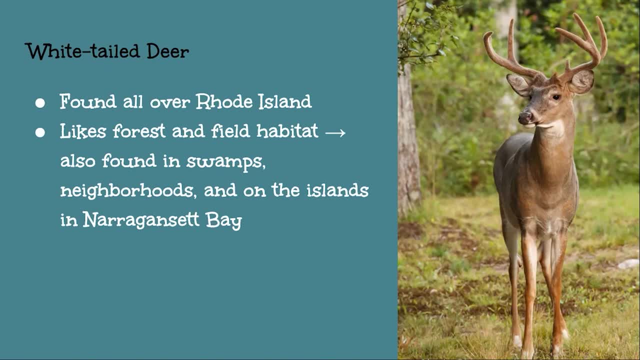 get into the game and absorb it. So we'll start with deer and then we'll go on to turkeys. So deer are found all over Rhode Island. They're in pretty much any habitat you can think of, primarily forests and open fields, but they also will hang out in swamps. They'll, of course, 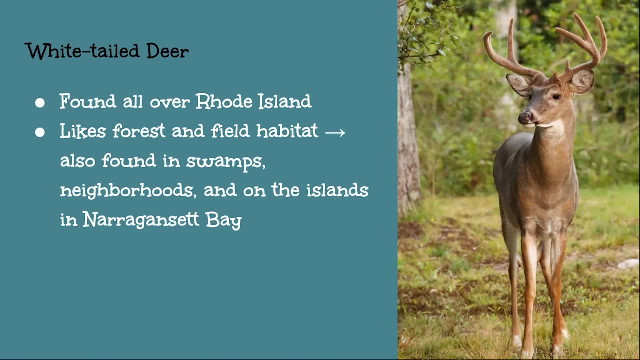 be in our neighborhoods. You know you're in the suburbs. you most likely have seen a deer wandering around in your neighbor's yards And even on the islands in Narragansett Bay, some of the closer islands, like Dutch Island, Prudence and Patience- the deer can swim out to those islands and they 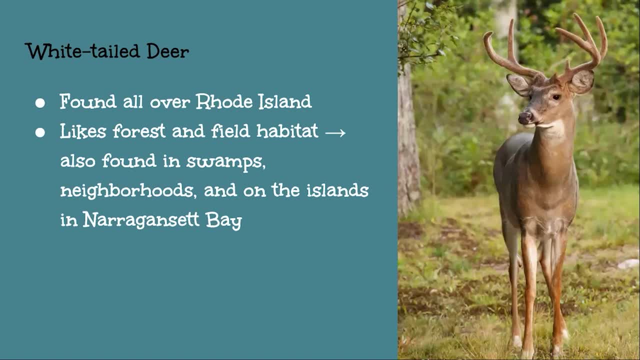 are very good swimmers Places like Block Island. there are deer there, but those were introduced by people. They were brought to Block Island so they did not swim there naturally, But because of that introduction and their inability to get off of them, they were brought to Block Island. 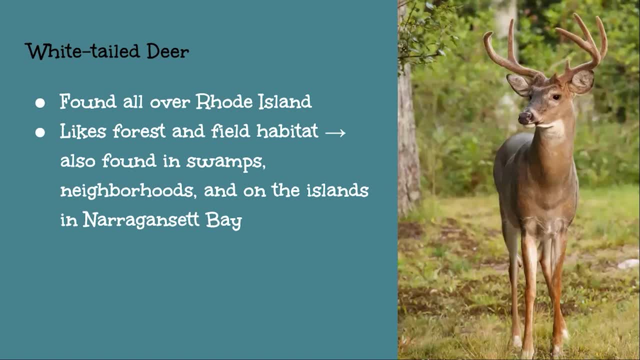 Whereas, like Dutch Island, they can go back and forth and go back to the mainland no problem. We have a major overpopulation of deer on Block Island. It's pretty densely populated. So that's a great example of what happens sometimes when humans interfere too much and it can explode. 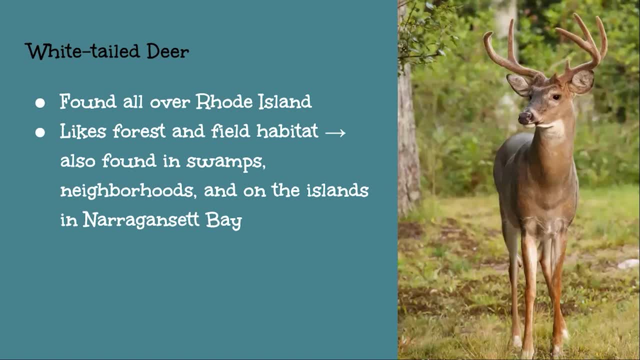 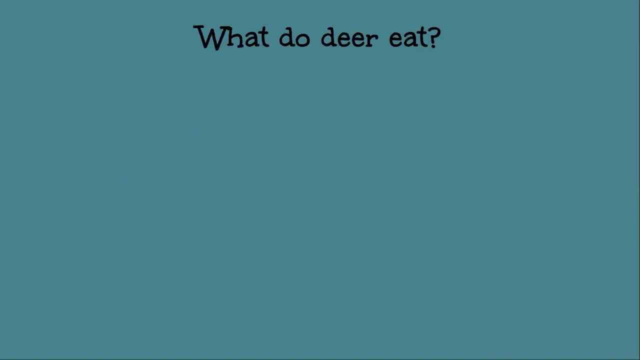 A population could explode And what are the ramifications of that on the health of those animals over time? What do deer eat? And this you know. the presentation is pretty interactive, so you can ask kids, you know, to come up with some ideas, write them on the board and have them answer. 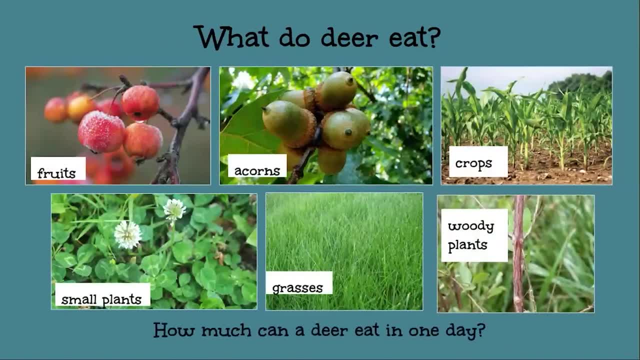 that question. So, in short, deer eat a lot of different things. They can eat 500 species of plants. They're not picky. They'll happily eat your garden flowers as well as all of these things here. So they're eating fruit. you know, naturally, that occurs out in the forest, but they'll also. 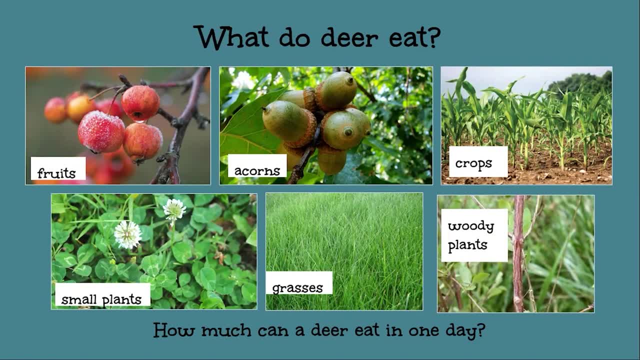 come into orchards and farms to eat fruit. there Acorns are particular. They're particularly important for deer, especially in the fall when they're trying to put on fat reserves for the winter, because food is very scarce in the winter So they survive off those. 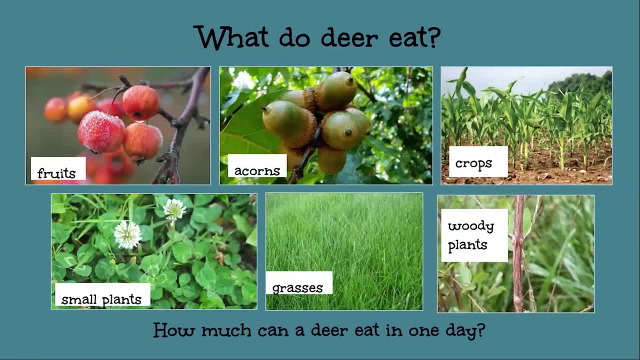 fat reserves and their metabolism slows way down. So all of those acorns are very, very important for them. So it's you know, when we have a good acorn year, then deer tend to do better over the winter, And some years acorns are a little sparse and that can affect how many deer survive over. 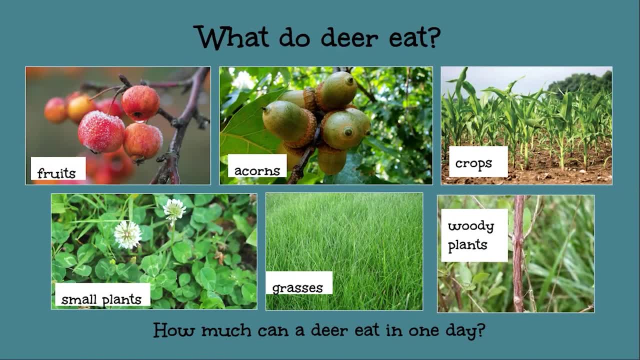 the winter, Of course, they'll go and eat crops, whether that's in your backyard, whether that's in your backyard garden or on your farm. lots of different small plants and grasses, and woody plants as well. You'll see deer snipping branches off of bushes and small trees- Any type of tree seedling. 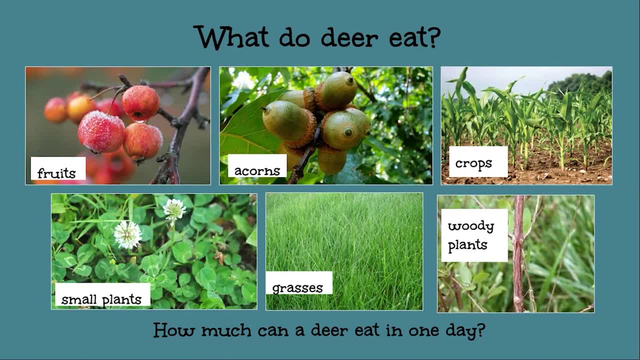 is very popular amongst deer, And deer can eat between five to nine species of plants, So they're very, very popular, And deer can eat between five to nine species of plants, So they'll go and eat crops, whether that's in your backyard. 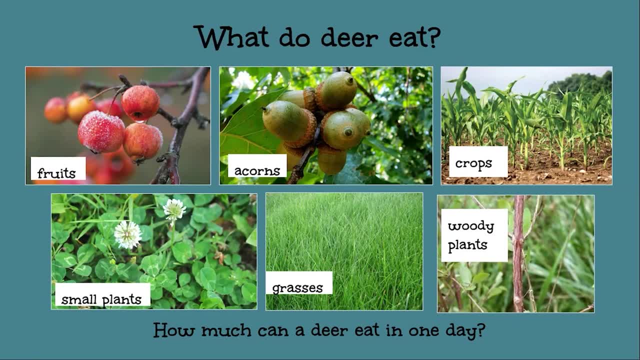 or on your farm. Any type of tree seedling is very popular amongst deer, And deer can eat between five to nine pounds of food in a day, So that's a decent amount of food. It's always kind of fun to have kids compare themselves to an animal Like: how much food do you eat in a day? Do you think it's five? 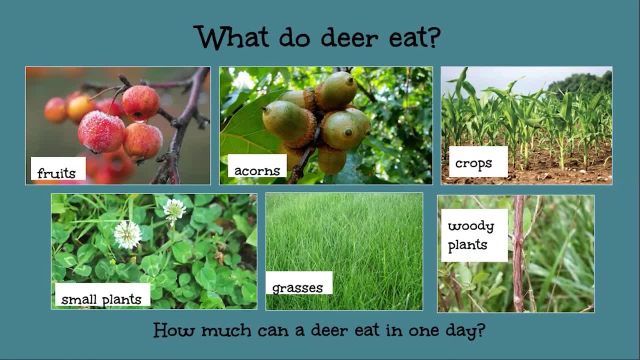 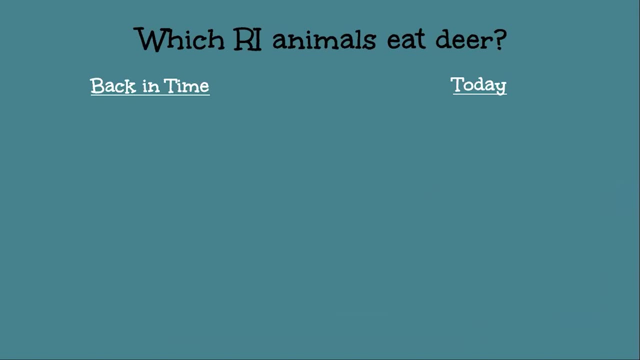 to nine pounds and maybe have something that weighs five pounds. Do you think you eat that much food in a day? Just to give them a perspective of how much deer need to eat to survive. So what eats a deer? This you know the answer to this question. 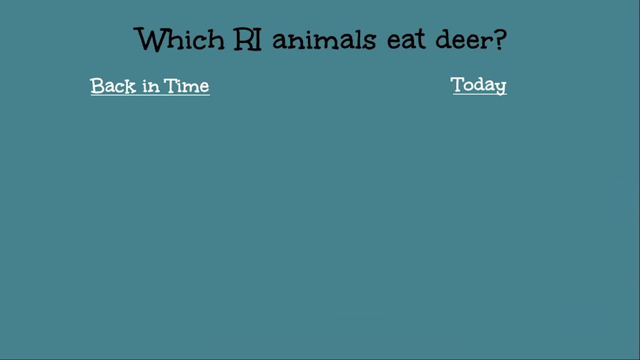 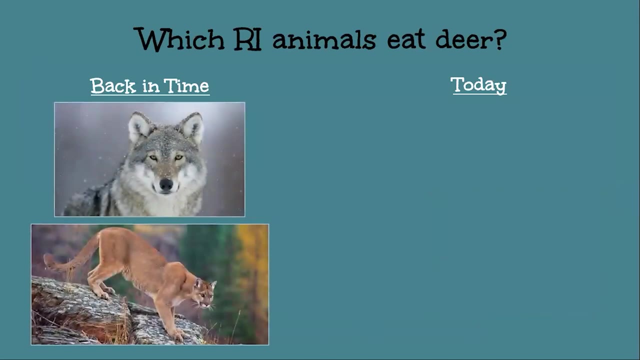 depends on when you're talking. So back in time and today, you know we have different predators for deer, because our predators have changed as we've learned in lesson one. So back in time we had mountain lions and wolves here that would prey on deer, And nowadays we don't have these. 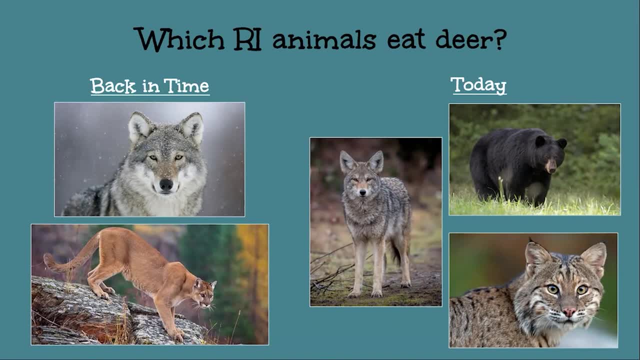 animals here in Rhode Island. So we have the coyote that will take out deer. You know they'll work together in a pack to hunt deer. Bobcats can actually take down deer in deep snow or they'll go for younger deer, smaller deer, And we have a lot of animals here in Rhode Island that are. 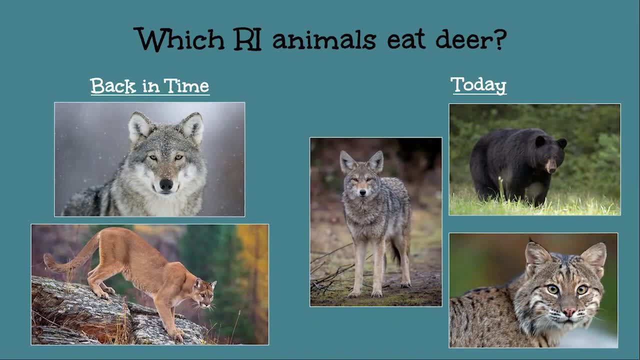 in deep snow- And bears occasionally might go for a fawn, or they'll eat carrion- If there's a deer that has died, they will snack on that and kind of garbage pick, so to speak. So these are all different predators that might be a threat to a deer and help keep our deer populations in check. 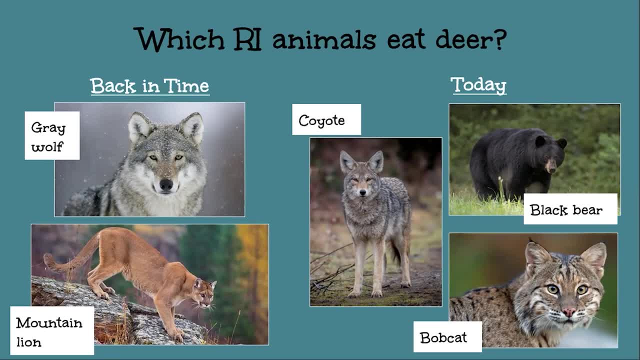 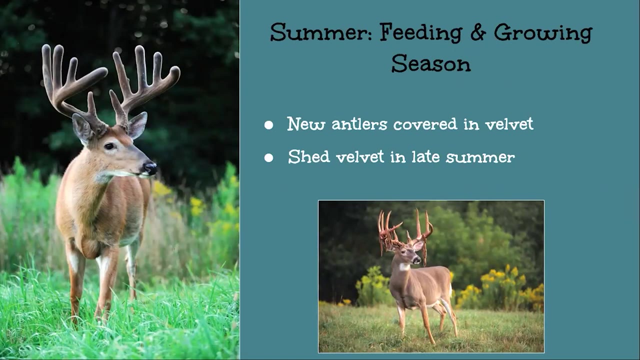 Predators are very important And especially in the turkey game. we do have a predator element in the turkey game to show how predators interact with prey species. So we have a few slides that go through the seasons with deer and what they're doing in a particular season, So in the summertime. 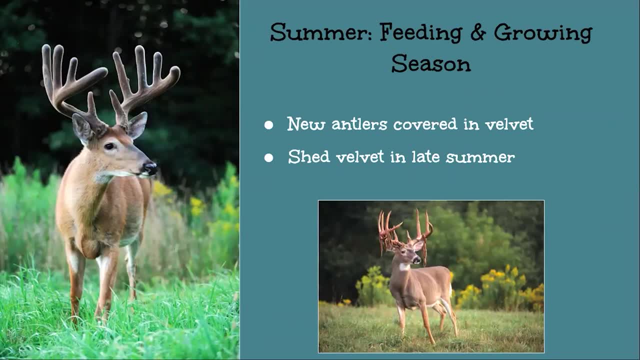 they're just focusing on eating and growing, So there's plenty of food around for them to eat and raise their young, And antlers will grow in the summer. So we have a male deer, a buck, here, who has a really beautiful 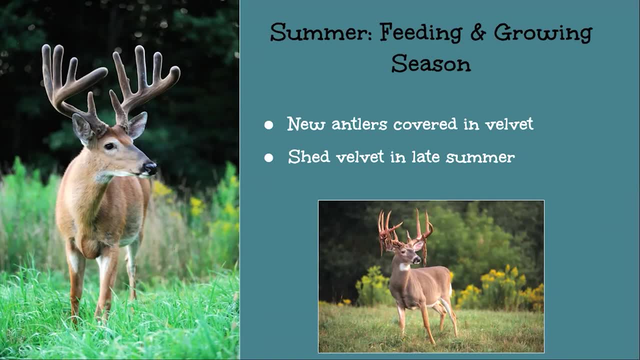 beautiful set of antlers And you can see they look kind of puffy and fuzzy. These are covered in velvet. So here in the notes we have a whole explanation of velvet and how it works. So this is living tissue, This is living skin, with blood vessels and hair on it And as the antler grows, 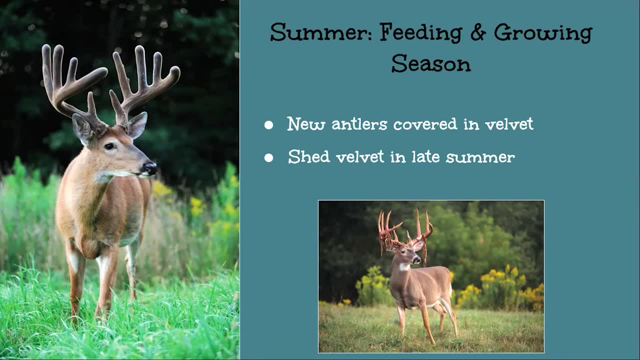 it's actually kind of spongy, So it's growing and there's lots of nutrients going up there, all the blood vessels and arteries and nerves that are building. So what we're doing is we're nourishing that antler And in response to the daylight hours, so you 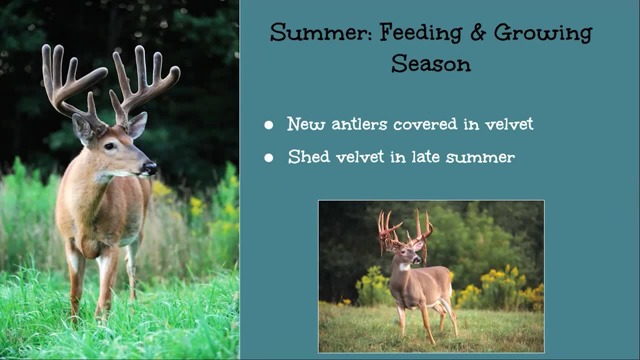 can see, as the daylight hours decrease, we start to see more testosterone production And then that triggers those antlers to turn from that spongy actively growing tissue into what we think of as an antler, as a hard bone, And then they'll shed that velvet. So this looks a little messy and a 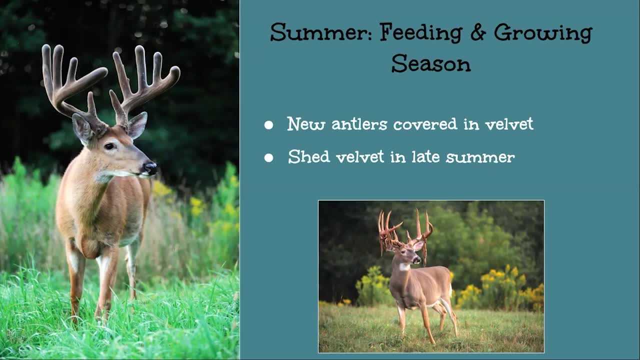 little gross here And you can see there's a tiny bit of blood. So that's from those blood vessels that were nourishing the antler's growth. So that's what we're doing, And then we're going to start to see the growth, And so bucks will lose this velvet at the end of the summer, And you might. 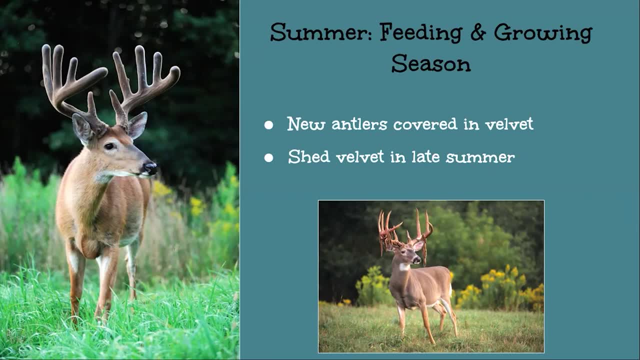 see them kind of scrape in their antlers up against a tree to kind of get that off. But it does fall off And then they'll have these nice smooth antlers going into the fall and winter And we have a really great. I mean, this is just a quick explanation of how antlers work, But we do have. 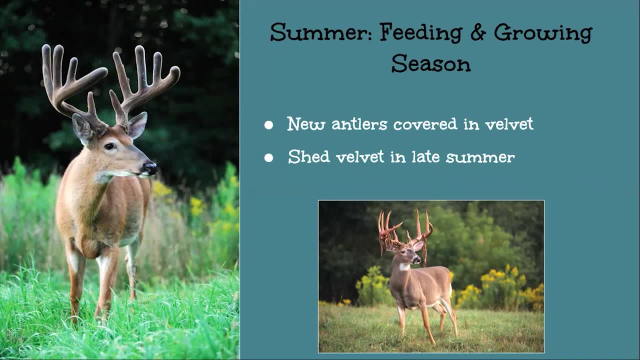 a really great article. So we'll go all the way down here. In our Wild Red Island newsletter we have an article that goes really, really deep into antler growth And it's a really, really in-depth with antlers and how this works physiologically to create antlers. It's really 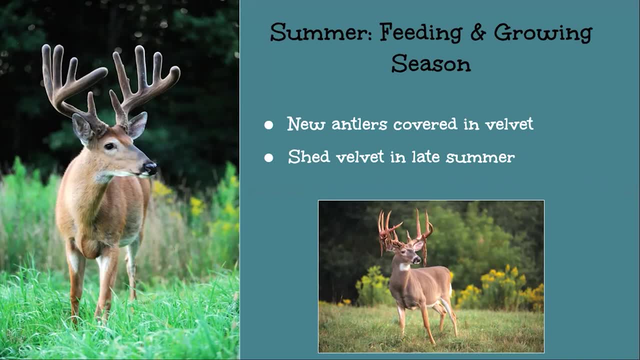 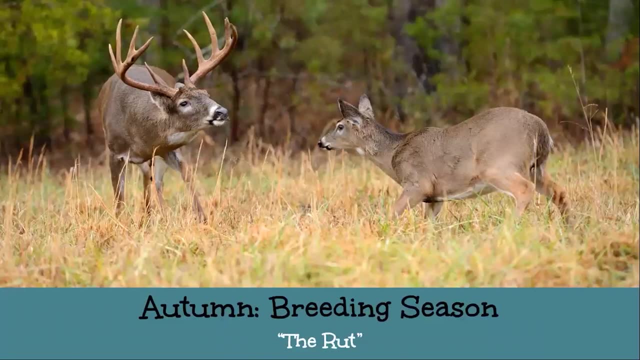 interesting. So if that's something that interests you or you think the kids have a lot more questions about, we do cover that here in the notes. So in the fall we go through the breeding season, also called the rut, And this is going to begin as early as September. But it's really 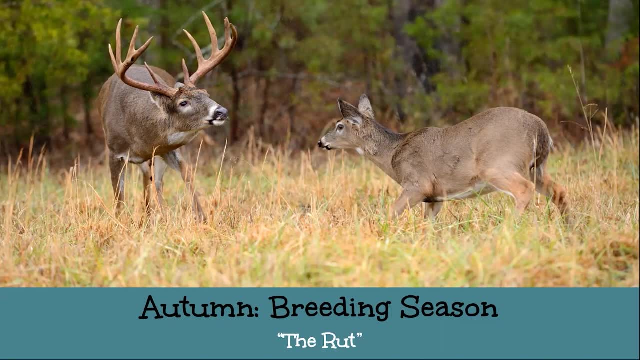 in November when it peaks And you'll see bucks traveling far and wide to try to find a mate. This is when we see increased collisions with cars, because they're just going across the roads and they're trying to their hardest to find a mate And during the rut, you know, they'll use. 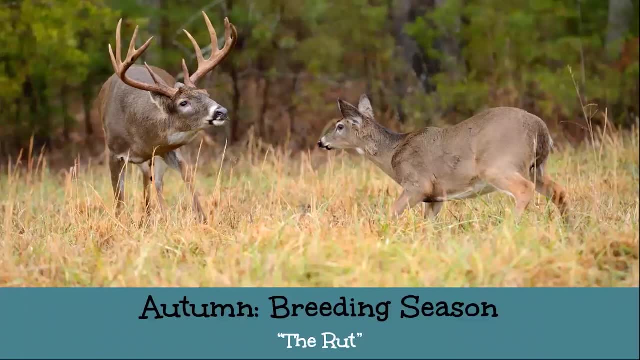 those antlers to tussle with other males and to assert their dominance over a territory. You can also find rubs on trees, So they'll take those antlers- the base of their antler- there's scent glands there- and they'll rub their head up against a tree to. 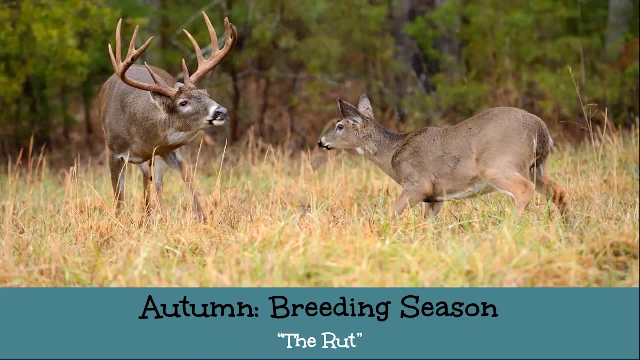 scrape off a little bit of the bark and mark their territory on small trees and saplings And they'll also create what we call scrapes. So they'll take oops a little too fast there. They'll take their antlers and kind of crash around with the branches. They'll take their hooves and 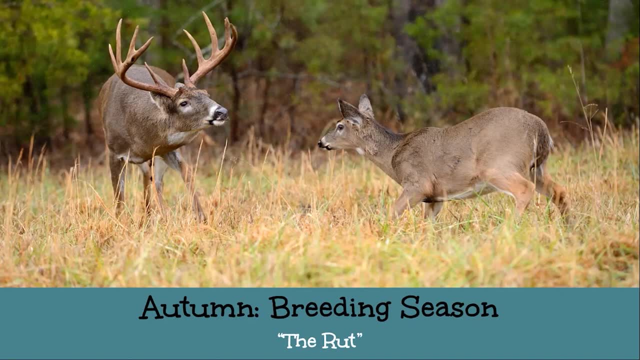 dig around on the ground, And those are all territorial signs like this is my area. Stay out, I'm looking for a mate. 007, 007, 008, 009, 0010. So we'll have the mating season during the late, early to late fall, and then we'll move into the 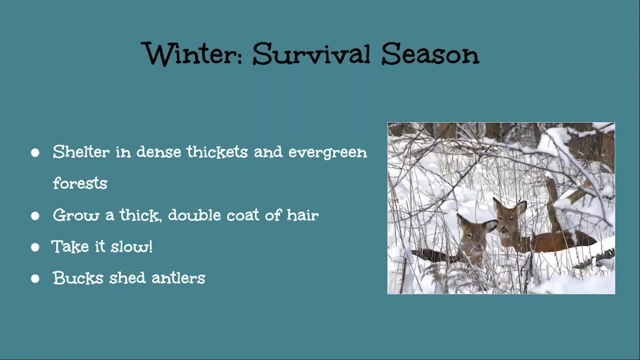 winter. So the winter is survival season and this is when bucks will shed their antlers. So this is a great time. you know, January and early January, late December is really great time to go out in the woods and look for sheds, because they'll they just drop, they drop off, nice and easy. 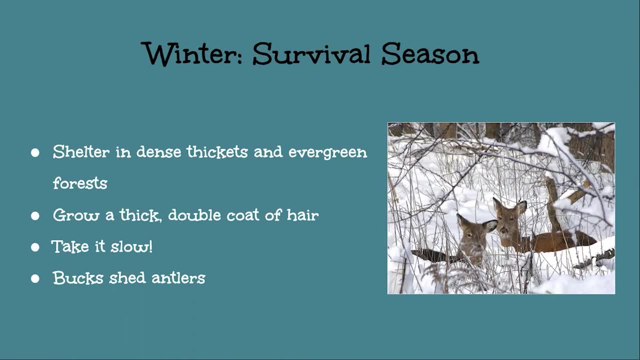 and there's a perfect break there. so they'll drop those antlers and focus on just surviving the winter. So you'll see deer bedding down a lot in the winter. they grow a double coat of hair, very thick coat of hair, to keep them warm and they'll they like to shelter in thickets. 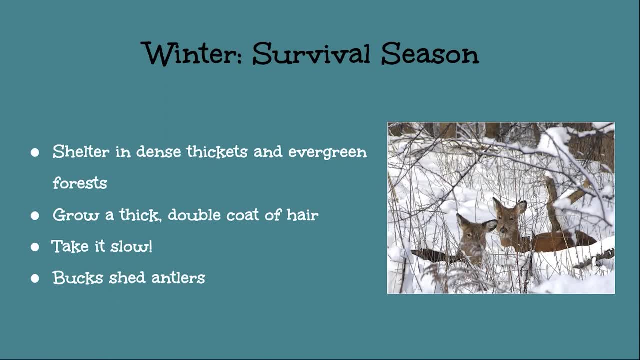 any type of pine or evergreen forest that gives them a little bit of shelter from the elements and it's really, it's really a rest and slow time for them. so their metabolism slows down and they're working off of those fat reserves that they've built up over the fall with the acorns and they just kind of take it easy. 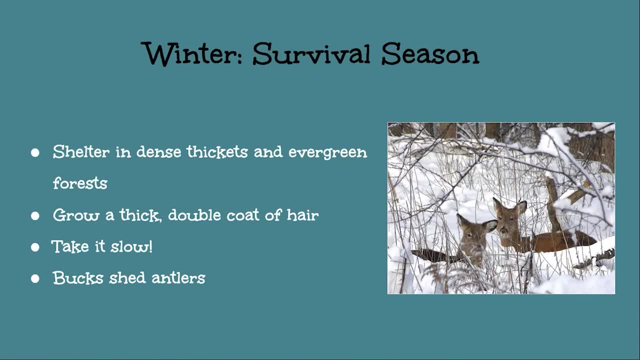 and they try to find whatever food they can, and we'll talk about you know, people like to try to feed deer in the winter and that's not really the best thing because of that slow metabolism, and we'll talk about that in just a second and how that can be detrimental to deer. 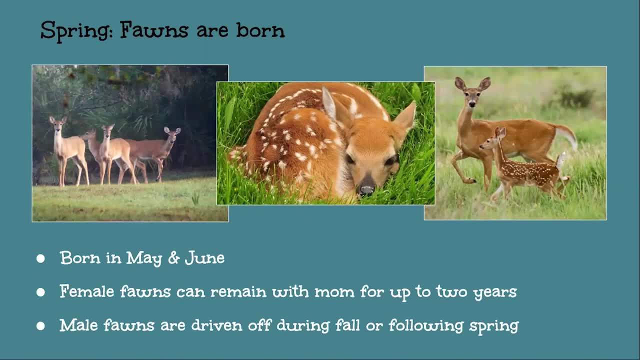 So in the spring they're coming out of the winter. you know going to try to put on as much weight as they possibly can and feed as much as they can. but fawns are born in May and June and they'll stay with mom for up to two years. so sometimes you'll see- you know a deer with. 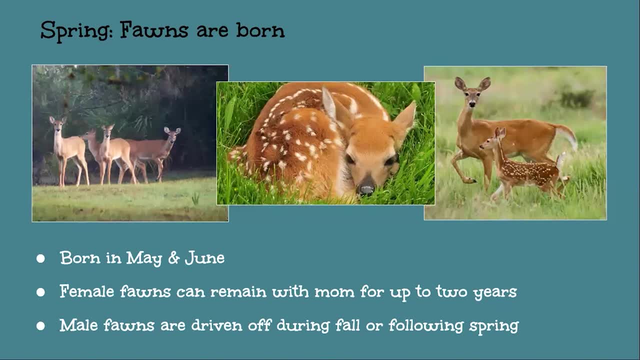 obviously you'll see them with a little spotted fawn, but you'll see them with a an adult doe with a smaller yearling fawn. so they'll hang out with mom for a little bit, but the males will mostly be driven off during the fall or the following spring. they don't stay with mom as long as the feed goes on. 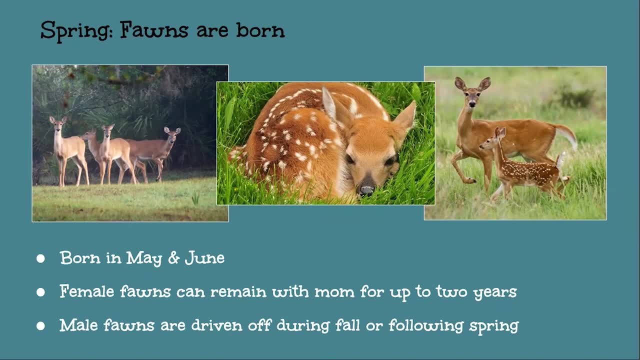 So they'll be born with these little spots and most of the time they just curl up in the grass and wait there for mom until they're able to actively follow her while she's feeding. but if you do find a deer, you know, tucked in your yard or anywhere, the best thing to do unless it's 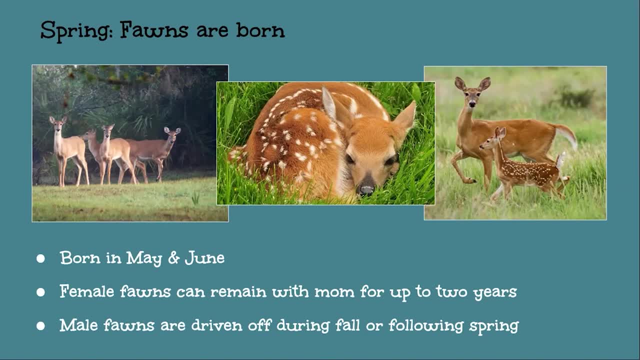 an immediate danger, you know, getting hit by a car or anything like that. the best thing to do is just leave it alone, because mom is nearby and this is their camouflage position: that they will not move. they are trying to look for food, are trying to lie low and and being close to a fawn will actually prevent mom from coming back. 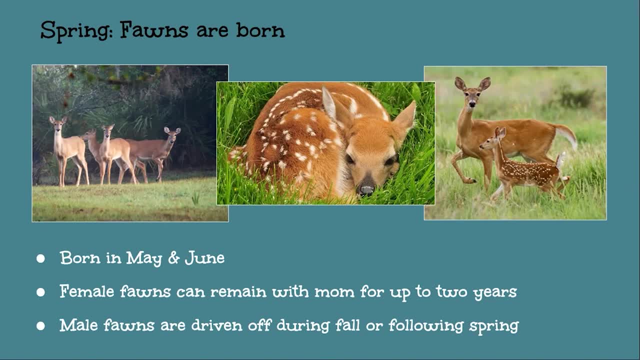 and feeding the fawn. she's going to be waiting for you- know, you, the predator- to disappear and leave the baby alone, because she doesn't want to draw attention to the baby. she's assuming that you haven't seen it yet. and it's? the longer we linger and the more we poke and prod at them, the longer. 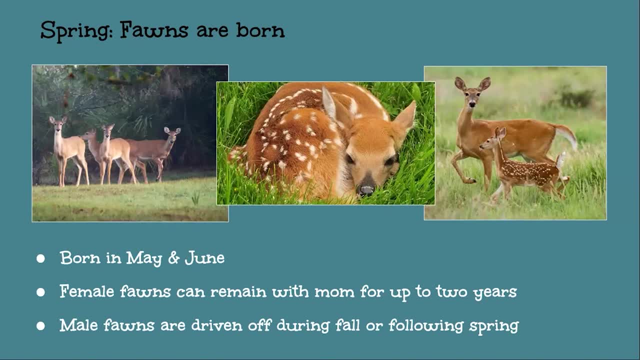 you keep mom away. so the best thing to do when you find a fawn like this, unless it's an immediate danger, leave it alone and just leave it alone and just back off and hopefully not to go back and check on it. you know a lot of people say oh. 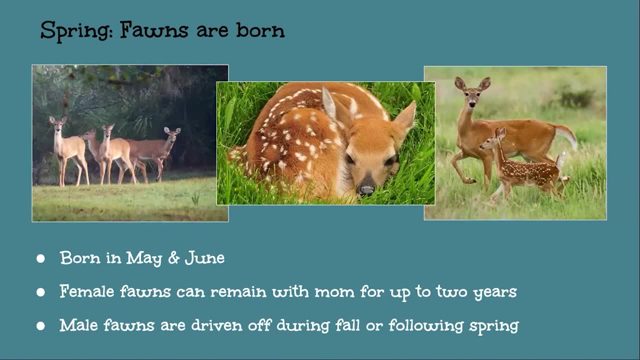 did the mom come back? you know, again, mom is watching. so making sure that you give them their space and not stressing them out is very important. um, so we do have some more notes. uh, about fawns you know in depth about. you know how they, um they could stand, you know, with an hour of. 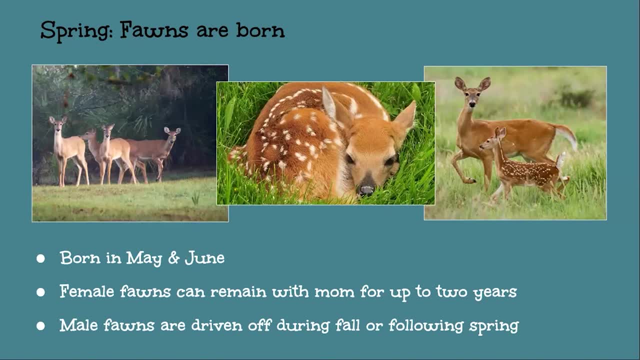 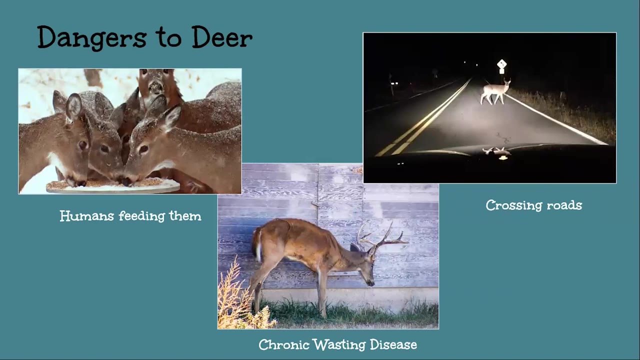 being born- um, sometimes does- can have twins or even triplets in some cases, depending on um. you know their nutrition levels, but for the most part they have one baby, uh a year. so some dangers to deer, you know. we've talked about crossing roads, of course, during 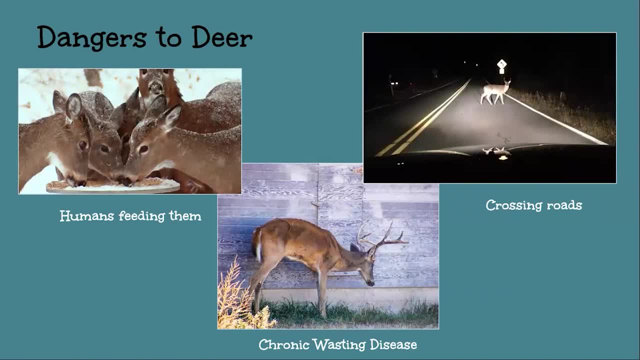 the rut. uh, humans feeding deer. so we have a lot of deer congregating here around a big pile of corn and, uh, it's. it's really really bad for deer to feed them, especially in the winter, because, um, you know they're- they're normally eating higher fiber food as opposed to 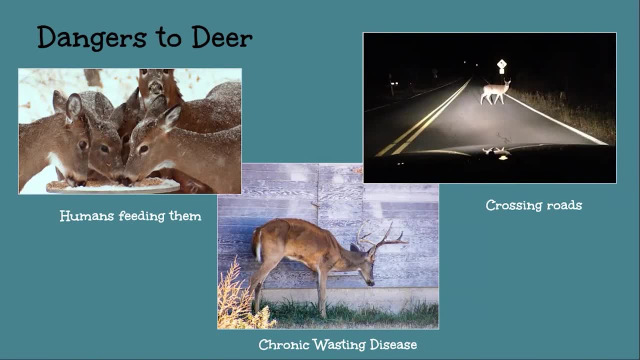 high carbs. so. so corn is really really high in carbs. and when you're shocking a system that has slowed down to just kind of rest over the winter and work off of those fat reserves, when you shock them with a bunch of carbs over and over and over again, it can actually lead to um disruption of 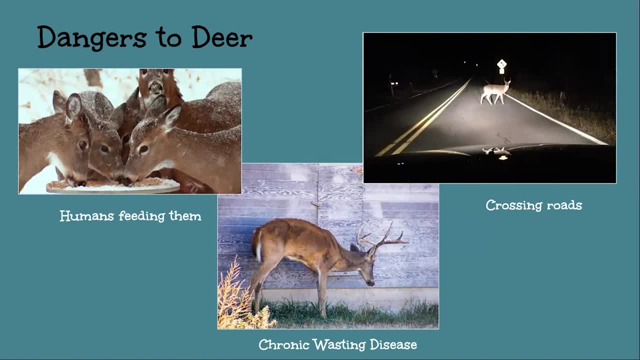 their digestive system and it can shock the system and it can even kill deer. so we highly, highly, highly encourage not to feed deer during the winter. it's technically against the law um to feed- intentionally feed- any wildlife in the state, with the exception of backyard bird feeders, um but putting out a pile. 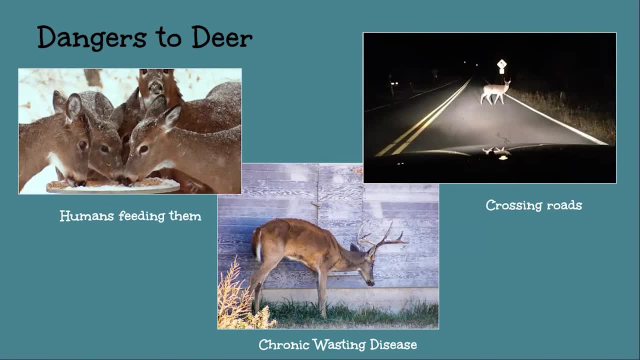 of corn for deer. it may seem like we're helping them. it may seem, uh, very kind and caring, and most people are just doing it out of you know, a kindness in their heart and they just want to help the animals. but the best thing that we can do is to not feed them because it encourages um. 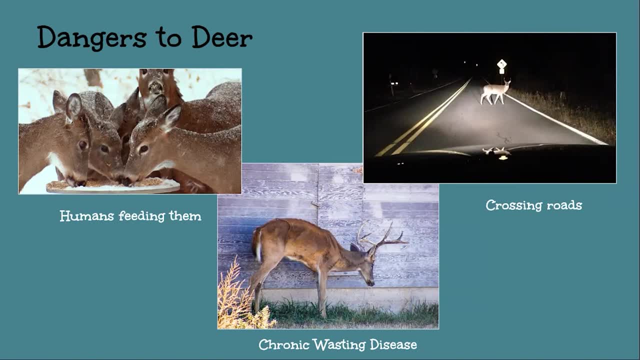 this, this type of behavior, also out of context, where the animals are just all over the place. it's not about feeding them now. there's so many different ways to deal with it and a lot of these, um- animal with diabetes, and so many of these animals in particular, are all hundreds of years old, all different types of animals, um, and it can be very. 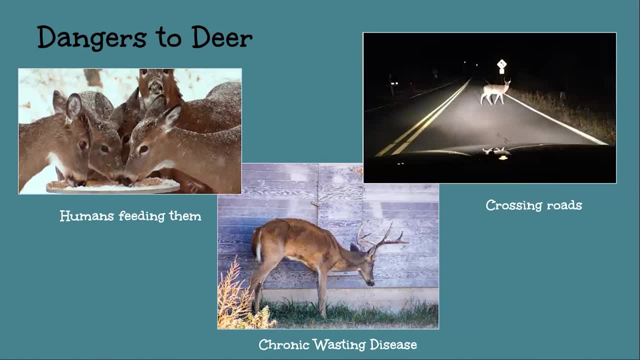 different when it comes to those animals. there is also a lot of looked at it, one number and, i think, disease. So we do not have chronic wasting disease here in Rhode Island yet, And that's a good thing, because it's a terrible disease. It's a neurological disease that affects the brain of the 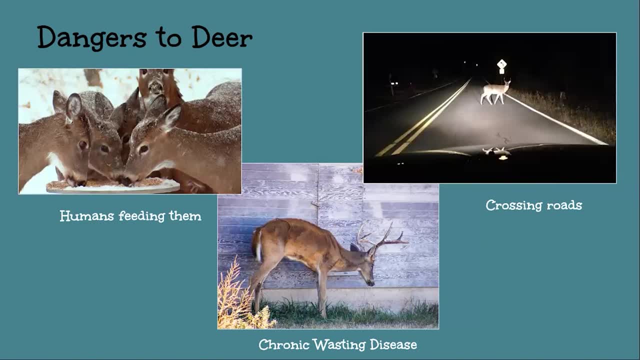 deer and it causes all of their muscle tissue to deteriorate, their brain deteriorates and they literally just waste away. So this is not a healthy deer And we'll see you know. if a deer has chronic wasting disease then you know it acts very differently than a healthy deer. They're. 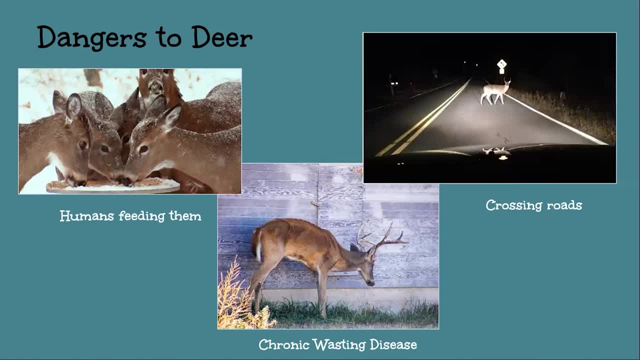 usually pretty lethargic and not looking too good. So we do not have that here, but it is pretty prevalent in captive deer facilities. It's, you know, in the Midwest pretty prevalent, And so it's escaped from captive deer facilities out into the wild and now wild deer are picking it up. It's. 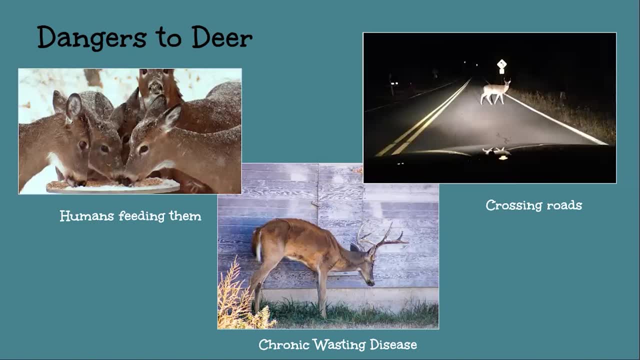 passed through urine and feces and also saliva, and it can live in the soil for a long period of time. So if a deer urinates, you know, here in the grass and it has the disease that sits in the soil for you know an amount of time. And if another deer comes over and eats, 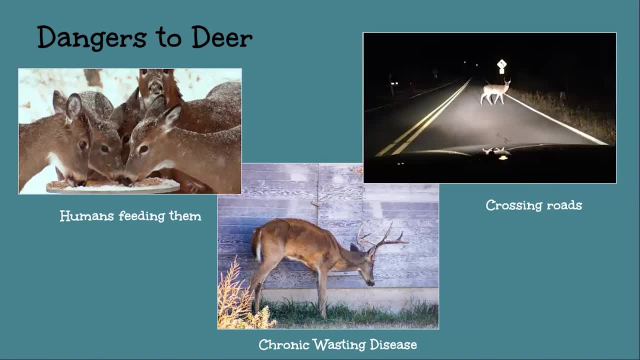 from this area, they can pick up that prion and get infected as well. So we do screen for this disease, which we'll talk about in a little bit. but this is a big problem in other parts of the country, So we're screening for it to make sure it does not get to Rhode Island and affect our 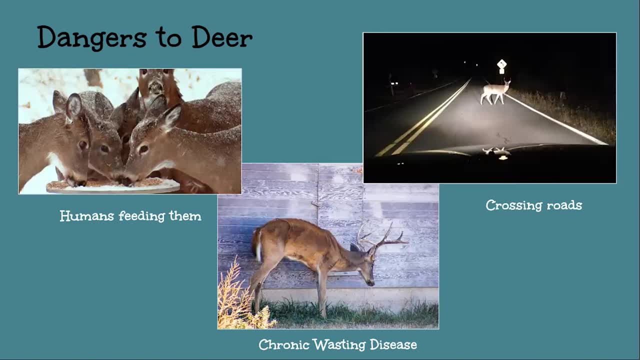 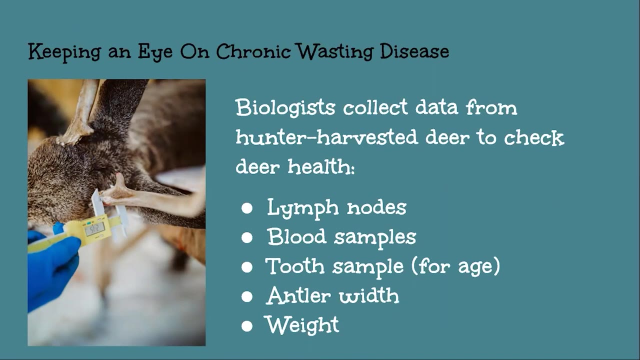 deer population. So that's again why you know, feeding deer passing saliva not a great, not a great idea When we're thinking about preventing this disease. So keeping an eye on chronic wasting disease requires a lot of data collection. So each year we collect data from hunter harvested deer. 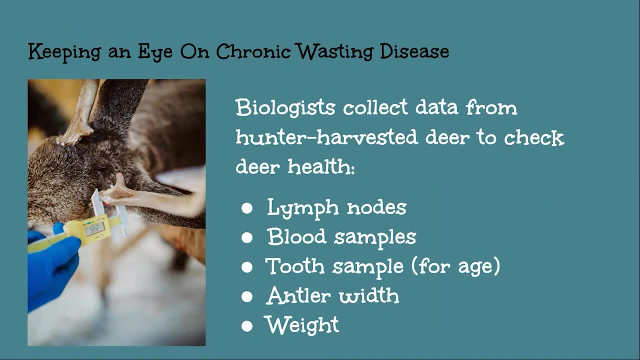 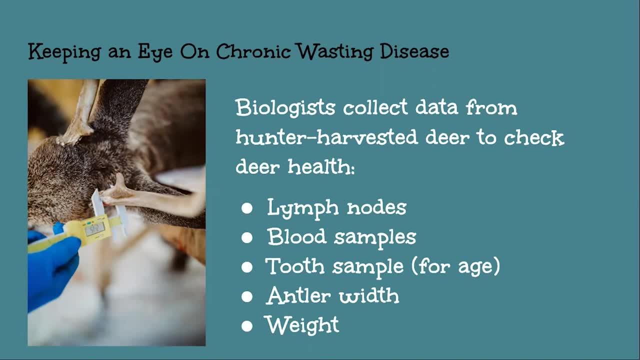 collect lymph nodes from deer, So those will be taken from either side of the esophagus. We'll take blood samples. we take a tooth sample to age the deer, because you can actually age deer. You can get a general idea of how old they are based on the wear on their molars, taking a look. 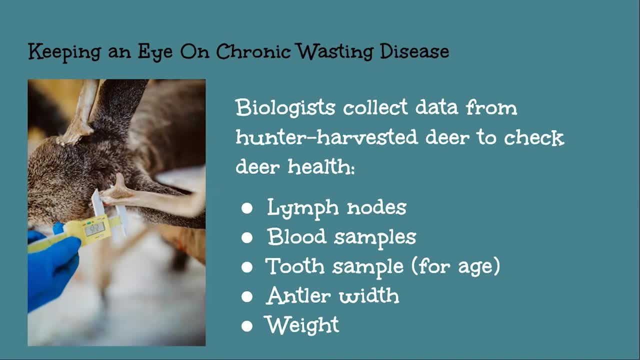 at those teeth and how much they've been worn down through the deer grinding their teeth to their food. But it's it's a relative age. So what we try to do is take a tooth sample, a lower incisor, send that to a lab. they'll do a core sample on that tooth to count the growth rings And 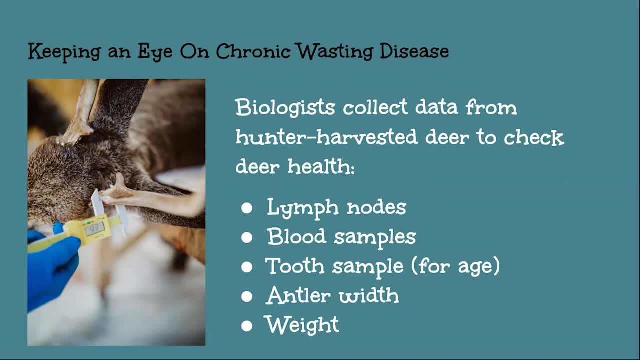 it's like growth rings on a tree And that's how they're able to determine the exact age of the animal. They'll also do an antler width and take a weight to try to just assess general health of the deer that have been harvested, And this is a really great way of how hunters can help us. 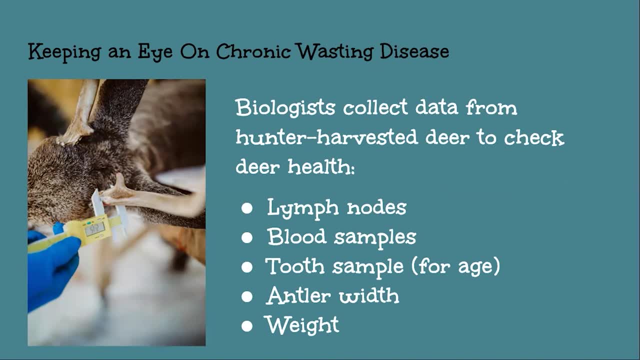 just monitor the health of our deer, And you know we'll do this, for if we get any roadkill deer, we'll also do that. We work with a number of game butchers as well, So throughout the season, not just during those check stations where hunters are required to bring their deer in- 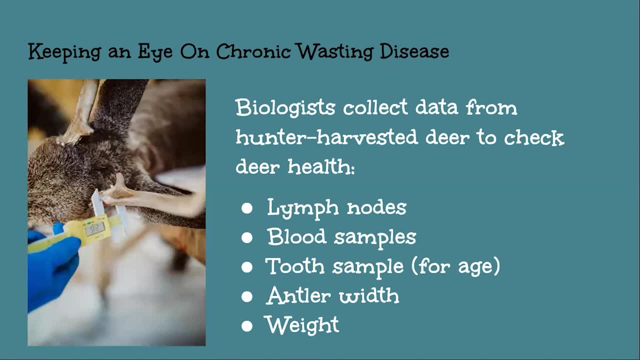 to be checked for those those four days, but throughout our deer season runs from September through the end of January, at least for archery. So we work with the game butchers as well to get more samples from archery harvested deer as well. So this chronic wasting disease is not just for 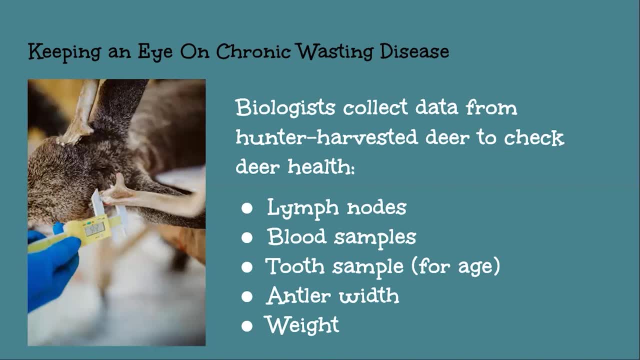 white-tailed deer. it affects moose and elk. So this is just a huge. it could be a huge problem for our, for our, all of our cervids, our deer species across the country. So this is very, very important that we monitor for it. So that's where 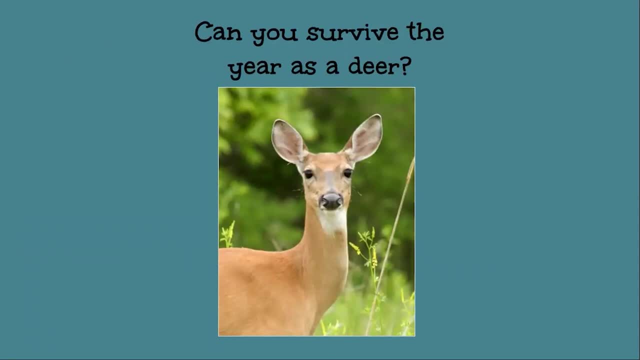 we would transition into the game Oh Deer and challenge students to survive the year as a deer. So they have to find resources to survive. you can introduce predators. you can introduce hunters into the equation. you can introduce predators. you can introduce hunters into the equation. you can introduce 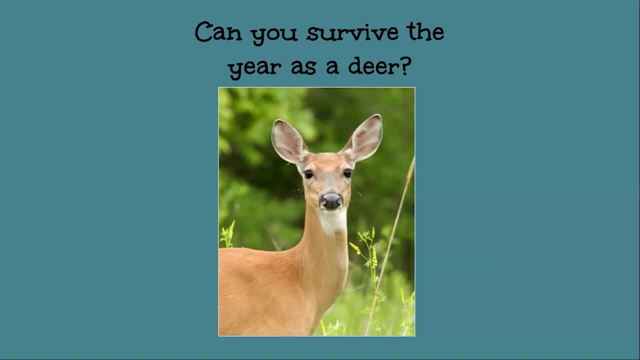 predators. you can introduce hunters into the equation. you can introduce hunters into the equation chronic wasting disease and how that spreads amongst the population. There's all different variations of the in the game within the the instruction packet for the game as well. So 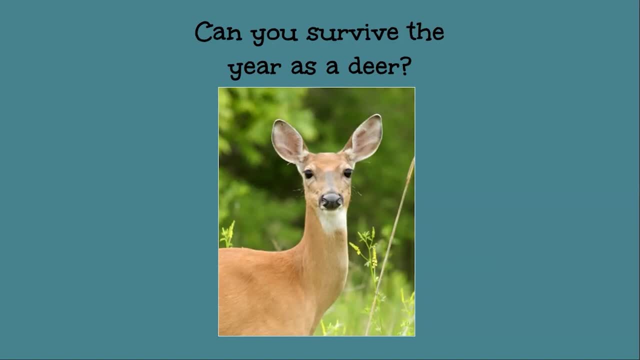 encourage you to get creative and have fun with it, And generally students get a big kick out of this game. It's a lot of fun to play seeing how their, how their resources and how all of those different factors will affect the population of the over time. 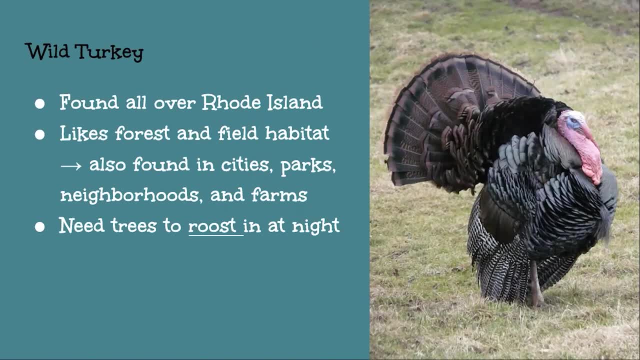 So let's jump to wild turkey. So turkeys are also found all over Rhode Island and they're also in forests and fields, but you can find them in cities and parks, neighborhoods, farms, But for the most part they really look for places that have trees to roost in at night. so roosting is just resting and sleeping. So turkeys can fly, believe it or not, they can flap and fly up into the tree and hang out there, and they're the primarily ground dwelling birds. they are ground nesting birds as well. 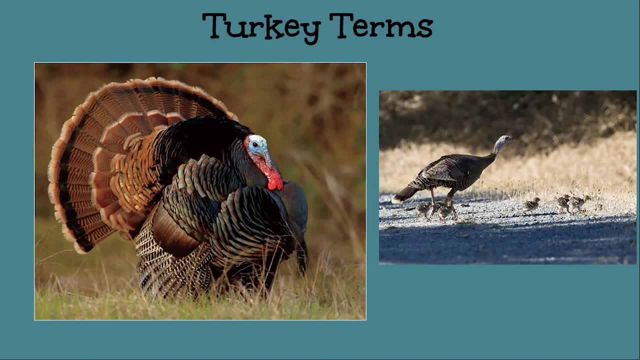 So we have lots of turkey terms that are very fun for students to learn. So turkeys have some really fun anatomical terms that you can have kids take a guess at. Some of them are a little different, So we have arrows that will go to all of the parts as well. So we'll start with a male. turkey is called a tom. 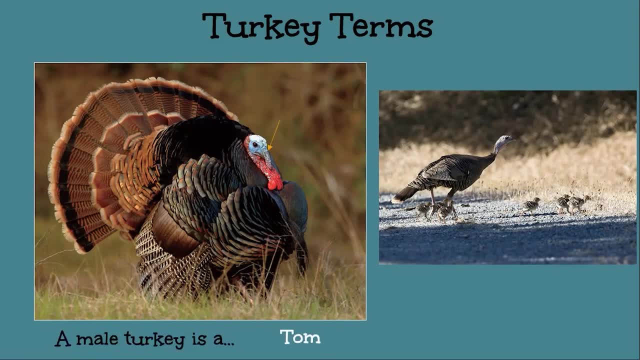 And we'll start to see all these little arrows pointing to things on the turkey. So we're looking at this little fleshy bump on the turkey On top of the beak. That's called the snood. We have these little bumps on the throat called the caruncles, and the snood and the caruncles- you can see that bright blue and red. So what the males will actually do is they pump extra. 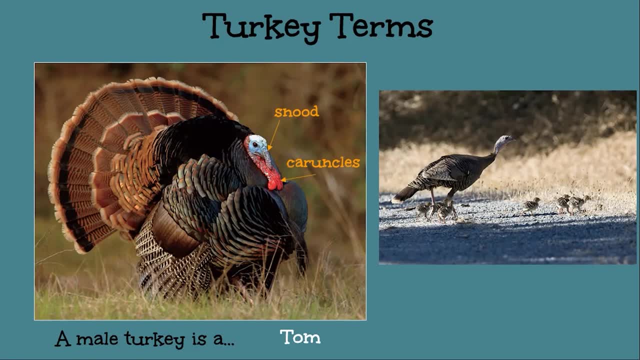 blood up into their face when they're doing this fancy fanning display so that will increase the vibrancy of the colors in their faces. they're trying to impress a mate And we have this little tuft of feathers right here that's sticking out. 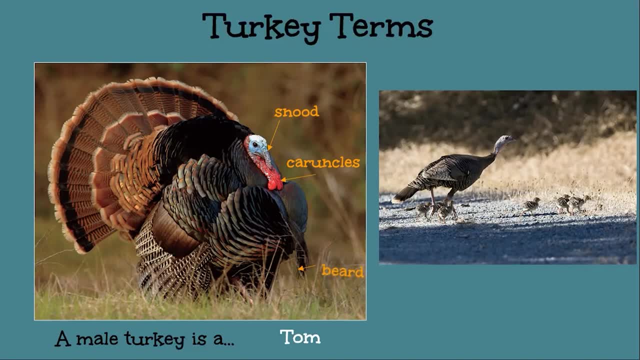 From the bird's chest and that's the beard. So typically it's just the toms who have beards, but you can see bearded females So which is a little little different. So when hunters go out and they harvest a turkey, they have to kind of use a lot of different clues. 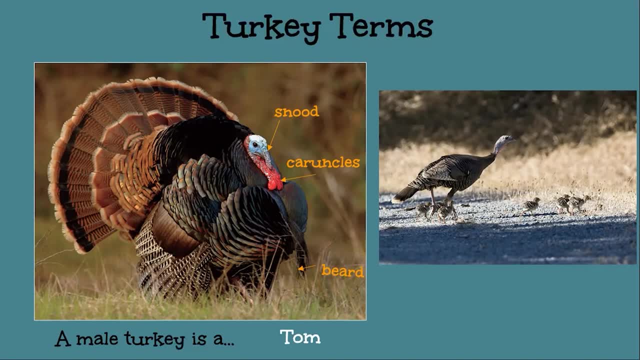 They can't just go on the beard alone to determine that it's a tom, because in the spring you can only harvest toms because the females are carrying and laying eggs and sitting on nests. So we want to protect them In the springtime and protect those broods. 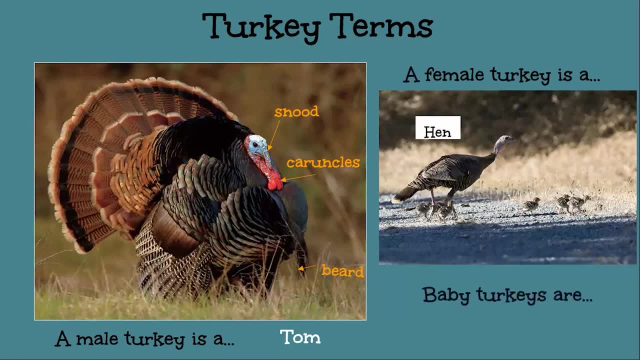 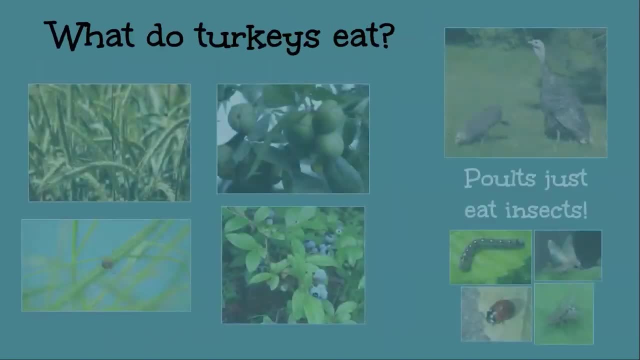 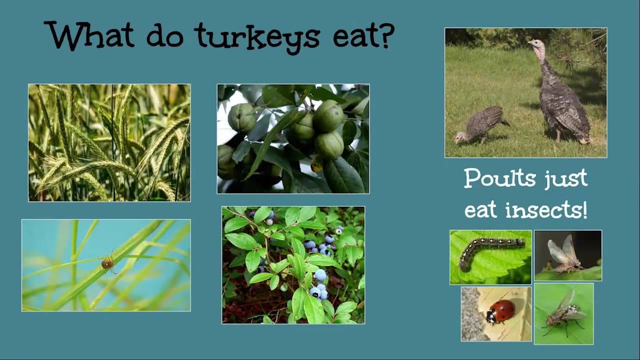 We have a female turkey is called a hen and the baby turkeys are poults. So again, similar to our deer slide. what to eat? lots of different things. So they're eating grasses and plants. They're eating fruits like blueberries, actually eat ticks and other bugs and insects. They'll eat snails. 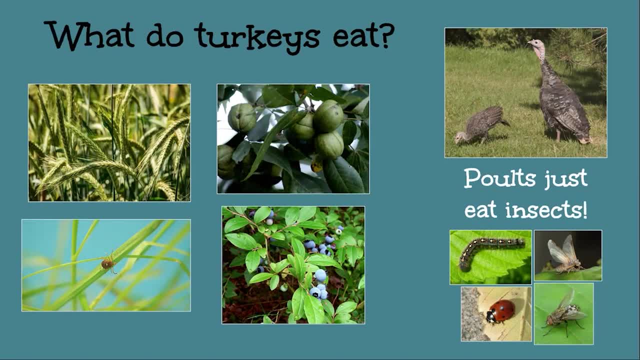 They'll have been known to eat salamanders and even hatchling turtles, if given the opportunity, and nuts as well. so beach nuts, hickory nuts, acorns as well. so acorns are not only important for deer, but also for turkeys as well. 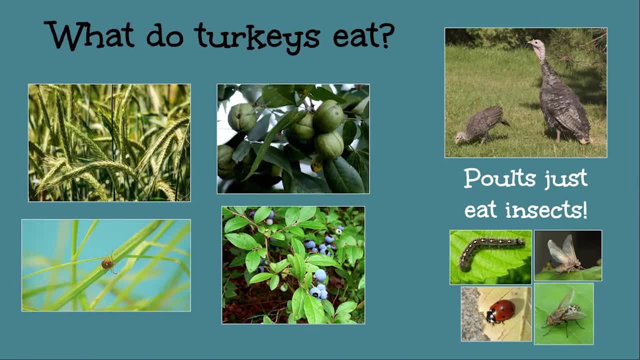 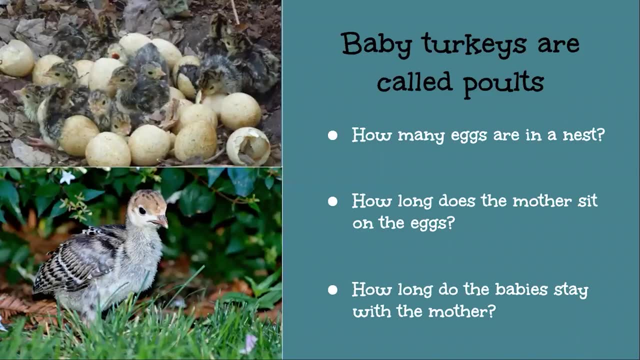 Poults survive solely on insects until they get to a little bit older, and then they'll start to eat all of the other items as well. So these little poults, you can see they're hatching right out of their eggs and you can see their eyes are open. 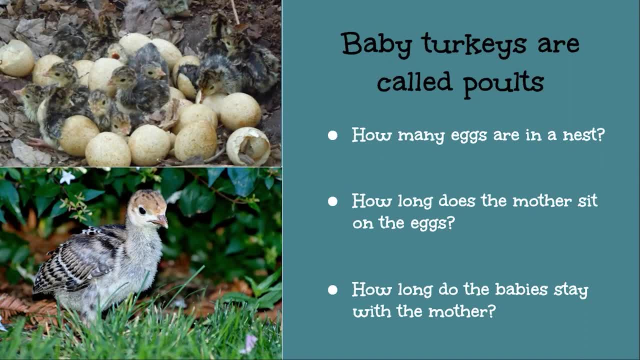 They're fully, full, Fuzzy and fluffy, Very different than if you've ever found a robin's nest. and you see, when the little robin comes out of the egg They're completely naked, their eyes are closed, they're helpless. baby turkeys are very different. they are because they're on the ground. the nests are on. 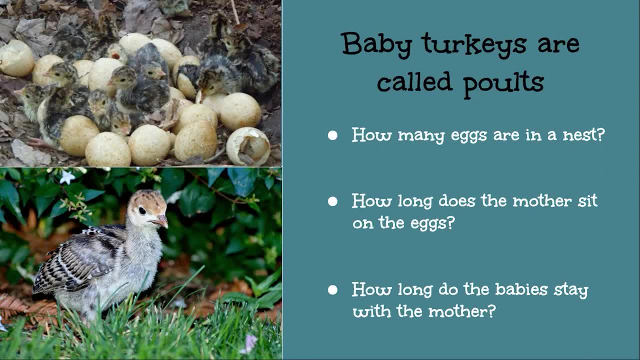 the ground. they're ready to walk very quickly because they have to be able to follow mom and and get out of their nest, because predators are lurking and able to pick them off. so they have to be able to stay with mom and keep up with her. 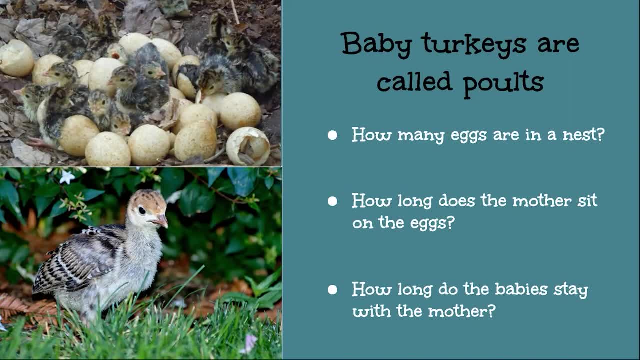 So they are very, very precocial and ready to go once they hatch. So fun trivia questions to ask kids how many eggs are in a nest. so they'll lay between 12 and 15 eggs and this is the nest. it's just a shallow depression in the ground. they're not doing anything. it was thick for twigs. 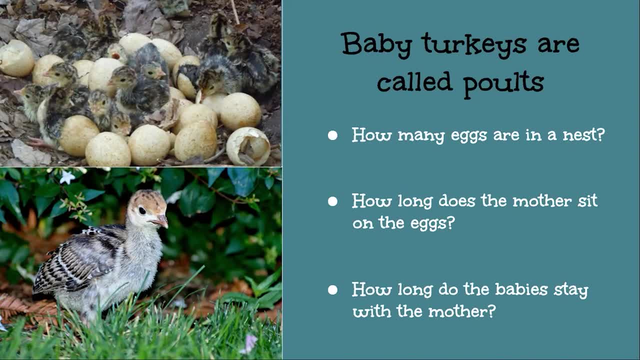 They're just relying on camouflage to have those eggs resting in the leaf litter and not causing a lot of attention to be drawn to it. How long does the mom sit on the eggs? So should be incubating those eggs for about 20 minutes. 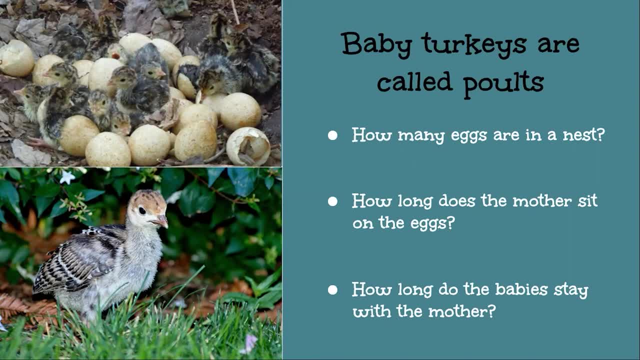 So should be incubating those eggs for about 20 minutes. So should be incubating those eggs for about 20 minutes, 28 days. And then how long would the baby stay with the mother? So we have about four to five months. Those poults will venture out on their own. You'll see them start to turn to these little. 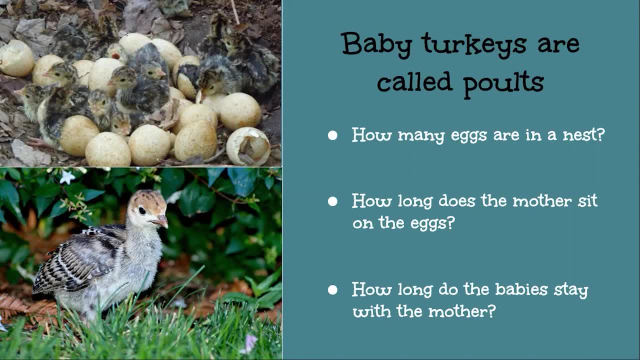 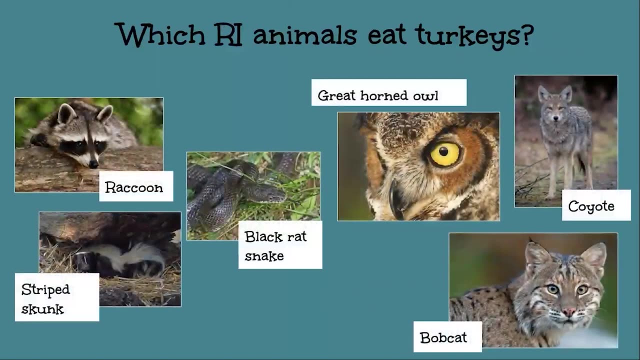 guys here as they get their feathers starting to grow. in those flight feathers You'll see them kind of getting a little bit bigger and bigger as the season progresses. So, similar to the deer, which animals eat turkeys? Lots of animals eat turkeys- Pretty much everything. 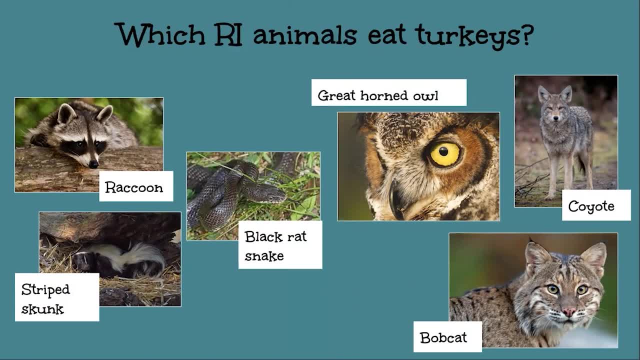 will eat a turkey, whether they're eating the birds themselves, either adults or poults- or they're going for the eggs. So raccoons, skunks, rats, snakes are notorious egg thieves and they'll happily eat those eggs out of the nest. Things like coyotes, bobcats. 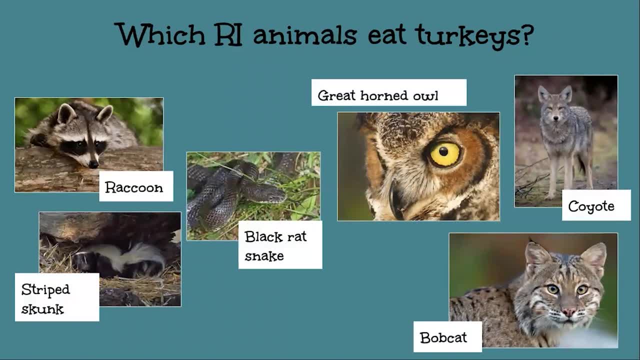 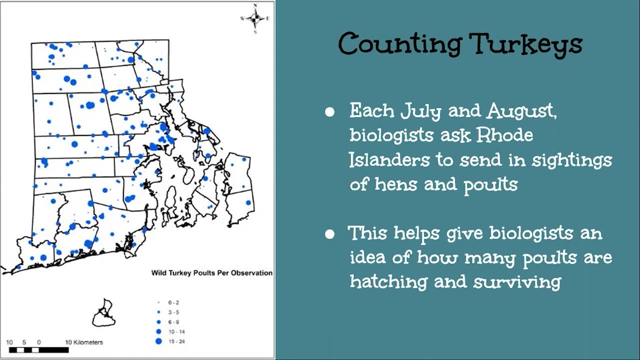 great horned owls will go for turkeys And then you'll see them start to get their feathers out- Adult turkeys and also poults, So counting turkeys. We also do monitoring of turkeys. It's a little different than our monitoring of deer, but this is something that students can get involved. 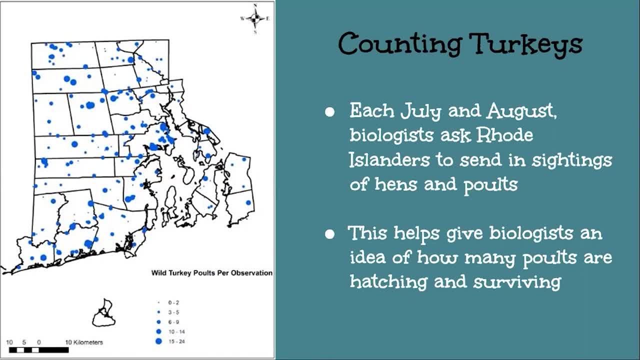 in and families as well. So each July and August we ask Rhode Islanders to send us in their sightings of hens and poults, And you can visit demrigov slash report wildlife to participate in that annual community science project And this gives an idea of how many poults are hatching and surviving throughout the state. So 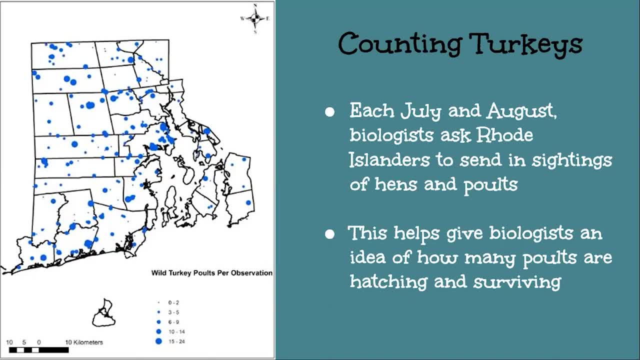 we've got our little map here with the bigger the dot, the more turkeys we're seeing in certain areas. So folks are reporting from literally all over the state in every town And that's a great way to gather data and showing that the community is just as important as our biologists in. 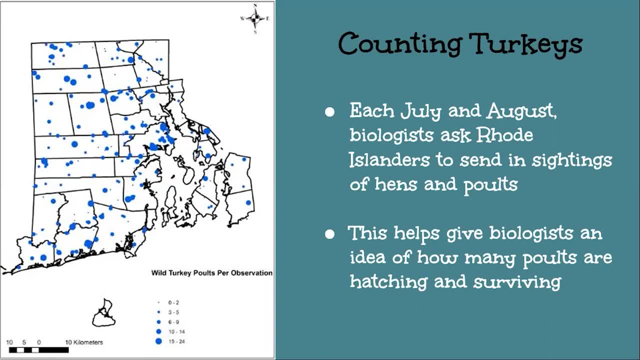 collecting that data, Because our biologists can't be everywhere at once and it's really great that we can rely on community data. And so we've got a little map here with the bigger the dot, the more the deer and the poults, And we also get a little anchor to do a focus on the deer survey And 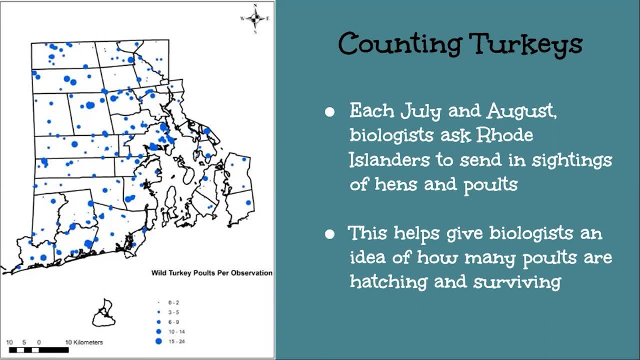 so we connect with our community members to send us those observations and help us collect that data. In this report, wildlife link- there is also a link to a deer survey that runs from August through September, as well as our herp observer survey, which allows you to submit observations of. 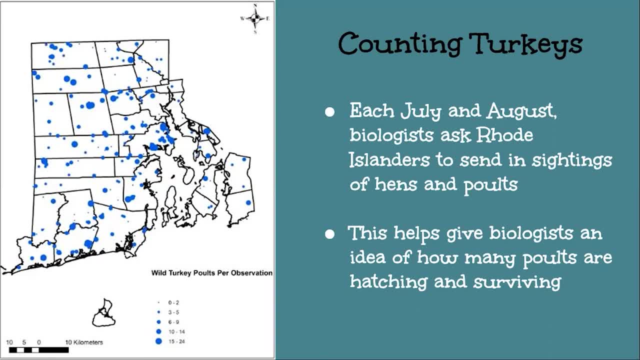 reptiles and amphibians any time during the year, So really great way to get involved and to be a scientist right in your own backyard. And then, of course, we would transition into the game Terrific Turkey, And if you have any questions, you'd love to be in the chat And I'll be happy to help you.